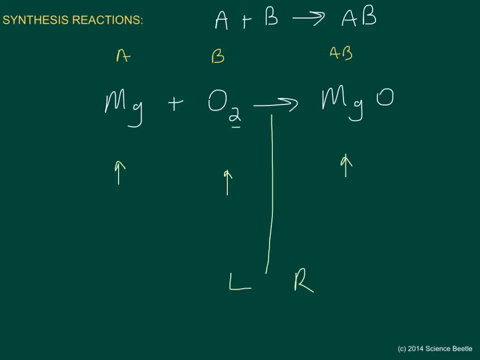 This little 2 indicates that we've got two oxygens on this side of the equation. So we look over on the other side of the equation and we notice that the magnesium oxide only has one oxygen. So what we are needing to do here is we need to add another magnesium oxide. 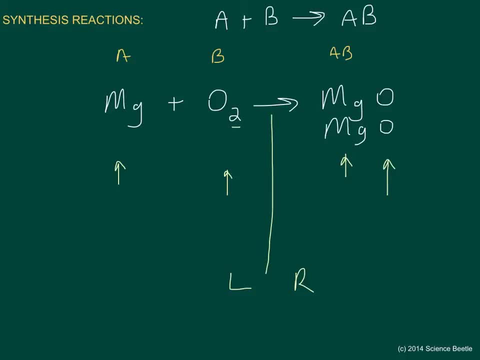 And what that will do is that that will bring our total oxygen count to 2.. But in doing so, yes, we may have balanced our oxygens, because now we have 2, but what we have done now is created a situation where we have two magnesiums on the right. 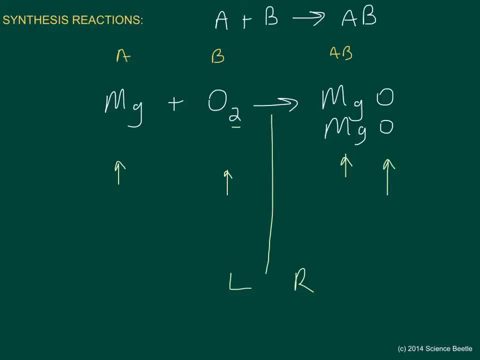 Notice, on the left-hand side we've only got one, So we are then required to add another magnesium to the left-hand side. If we do that, what we've got here now is a total count of our magnesiums here of 2.. 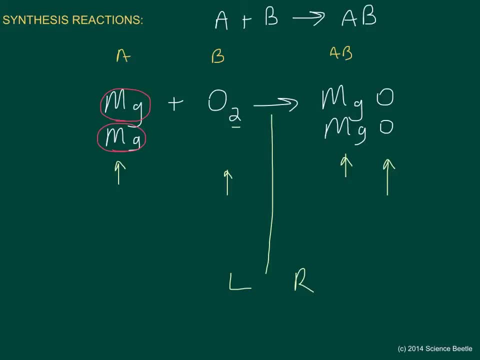 Notice we've got one unit, two units. So then we're going to have to add a coefficient at the front of this magnesium, indicating that we've got 2 moles of magnesium. If we turn our attention to oxygen, we notice we've got one unit there, or rather one mole of oxygen. 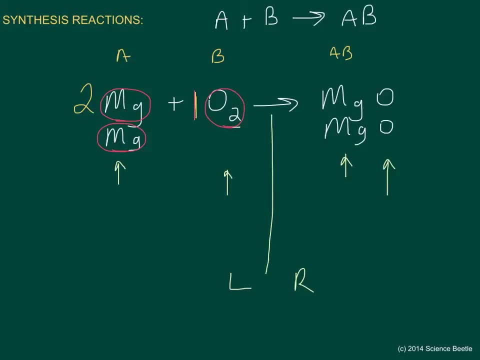 And so let me change that in To this color. we've got one mole there, And if we look at the magnesium oxides on the right-hand side, we've got one, two units there, indicating that we've got 2 moles. 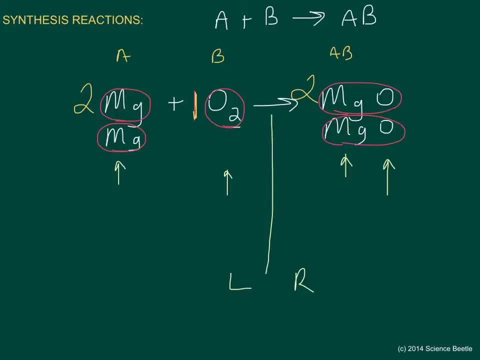 So if this were a problem that you encountered, say, on a quiz that's multiple choice or an exam that's multiple choice, what you want to do is you want to go ahead and look for the answer that provides you the following coefficient number: 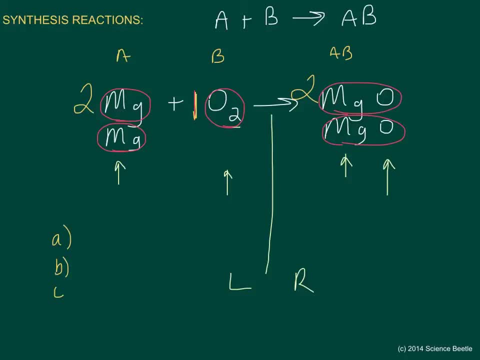 Maybe. perhaps you've got like an A, a, B, a C And I'm not going to write these out, but let's pretend that our answer for A actually said 2, 1, 2.. This would be the right answer because essentially, the 2 here is the 2 that we identify there. 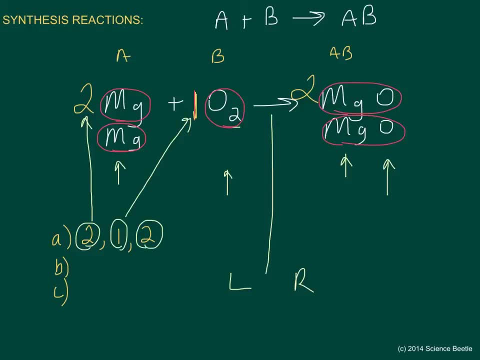 The 1 here is the 1 identified with oxygen, And the last 2 is identified with the mole number for the magnesium oxide on the right-hand side of the equation. So this is the first example of the 2 that I was going to provide you. 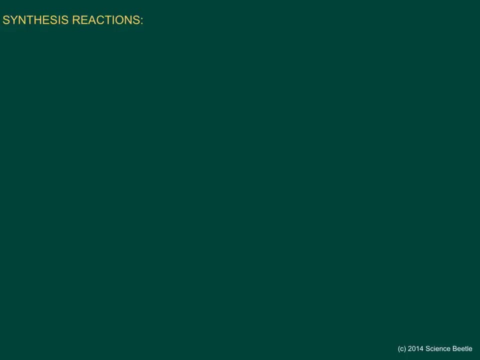 Let me go ahead and show you another example. Okay, so we'll begin again. I just cleaned the screen for us, But again, let me just write what we know. We know that A is going to react with B and that's going to form compound AB. 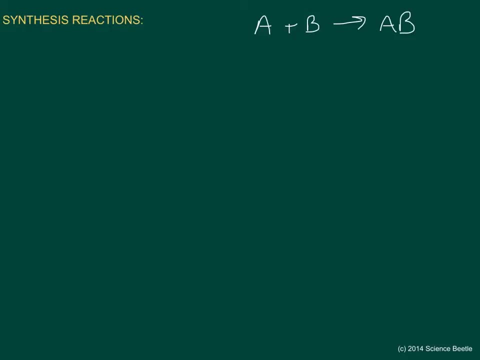 All right, so here we go. The second equation that I want to show you is the following: Let's say that we have iron, and so iron is going to be Fe, And Fe reacts with oxygen to form FeO. Now I could make this a little bit more complicated and kind of tell you: 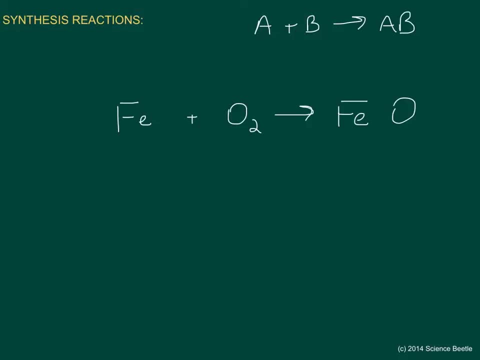 try to figure out what is the subscript for the FeO on the right-hand side. But what I'll do just to make this a little easier for us. I'm just going to tell you that it forms a compound where you have 2 atoms of Fe. 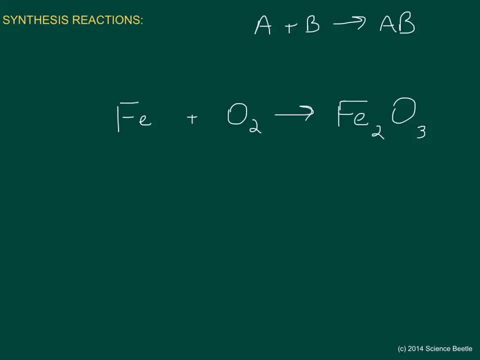 and 3 atoms of oxygen for this compound. Okay, and so our job now is to identify how we go about balancing this equation, And we first begin by writing the line in the middle, left and right, And we do this at the arrow that indicates that that is the middle point. 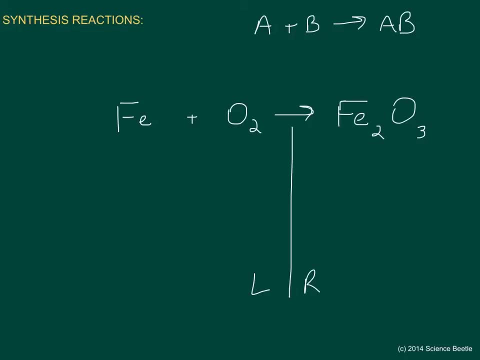 or the line that divides the left and right. And then I begin by looking at my iron. on the left-hand side Notice I only have 1 iron, and we can see that here, And on the right-hand side notice I have 2.. 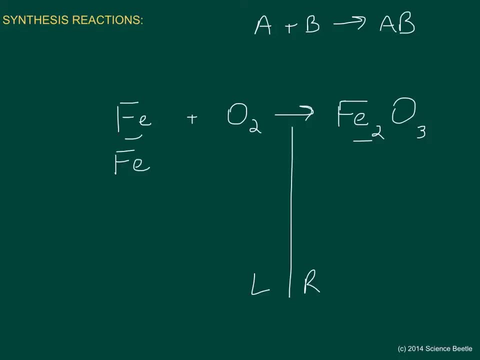 So I would need to add another iron to my left-hand side, which I'm going to do now. Now I've got 2 irons on the left, 2 irons on the right, So then I can move to the next atom on the left, which is the oxygen. 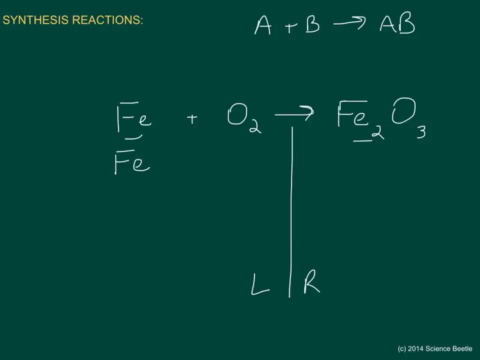 And I've got 2 oxygen atoms on the left, But on the right I've got 3.. Now this is a situation where you notice that this subscript here is odd. The first thing that I would be inclined to do is to just go ahead and add another compound of Fe2O3.. 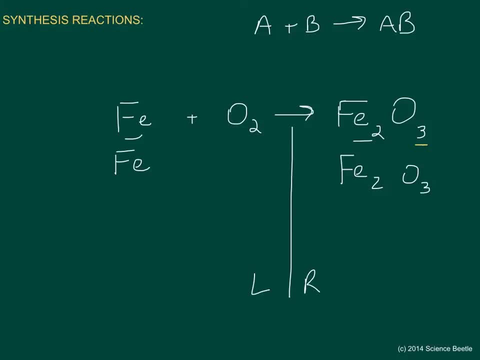 And if I do that, notice that now my total oxygens is even, because 3 from the first one and 3 from the second one gives me a total of 6 oxygens. Now, once I've done that, I've increased my iron count to a total of 4 on the right: 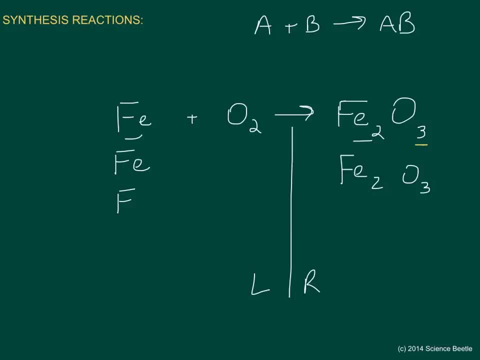 which means I need to come back over here to the left-hand side, and I need to add 2 more, And so now I've got a total of 4 irons on the left, 4 irons on the right, And now all that's left to do is to balance out my oxygens. 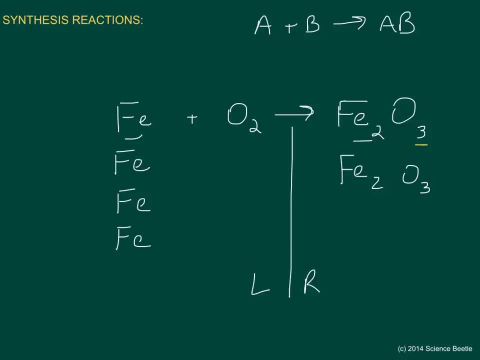 So I begin with the oxygens on the right. I've got 6 there and you can see that here- 3 and 3, that'll give me a total of 6. And I've only got 2 on the left-hand side.